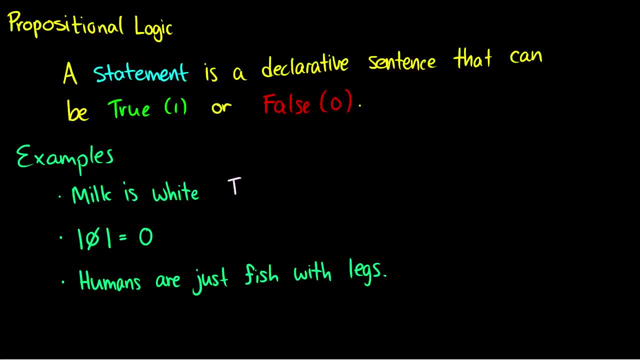 the cardinality of the empty set is equal to 0. That is also true. so that is a statement. It can be true or false. And finally, humans are just fish with legs. Well, that's not true. We are not fish with legs. We're much more than that. 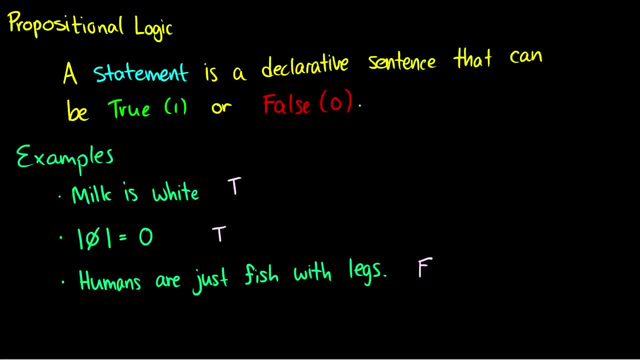 so that's false. But the point isn't whether or not these statements are true or false, but rather that they are statements, which means that in propositional logic we can express them. We cannot express things like questions, So, for instance, questions cannot be true. 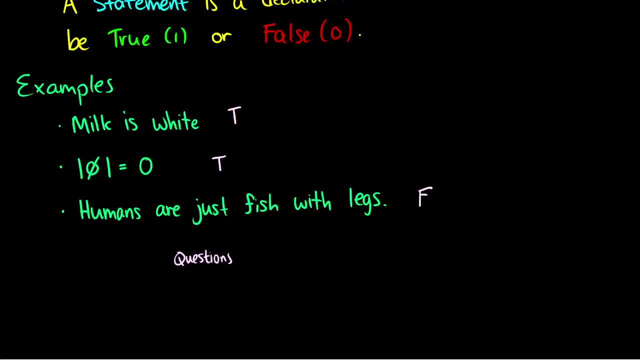 or false? Will you go to the store? for me, True Doesn't make any sense. The other things we can't call statements would be imperatives. So imperatives are not statements. What is an imperative? An imperative is a command like kick me or kick him. Those can't be true or false. 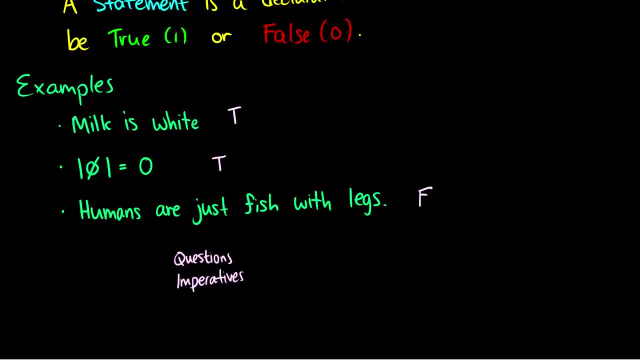 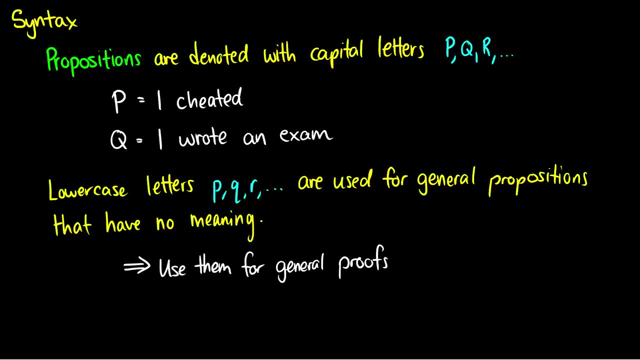 So when we talk about propositional logic, we're dealing with statements which are true or false. So the syntax of propositional logic Use the word propositions. here, Propositions and statements are very closely related. A statement is usually a very specific instance, while a proposition just captures the general idea. 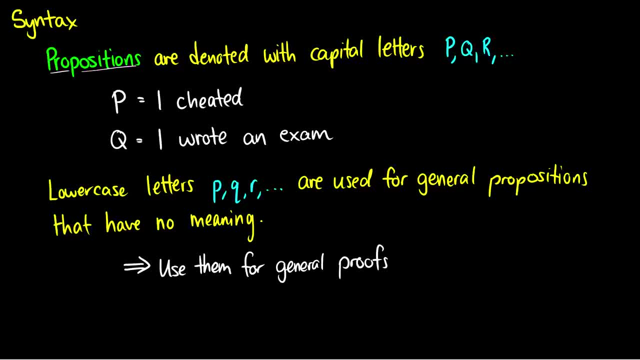 of a statement, But for this course that really doesn't matter at all. The distinction isn't important. If you're a philosophy of logic instructor or a student, then it might be a little bit important to distinguish between the two. But propositions or statements are going to. 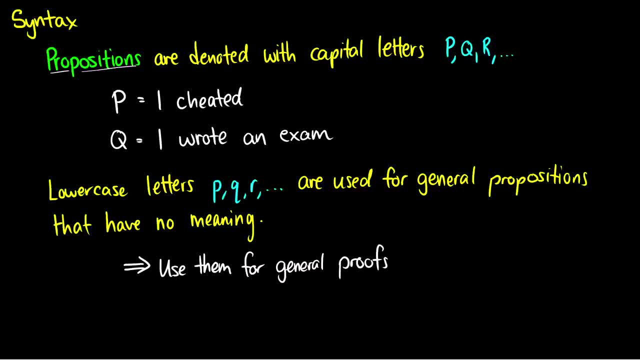 be denoted with capsules. So if you're a philosophy of logic instructor or a student, then you're going to be denoted with capital letters like PQR. So, for instance, P is I cheated and Q is I wrote an exam. So those are propositions. Lowercase letters P, Q and R are just. 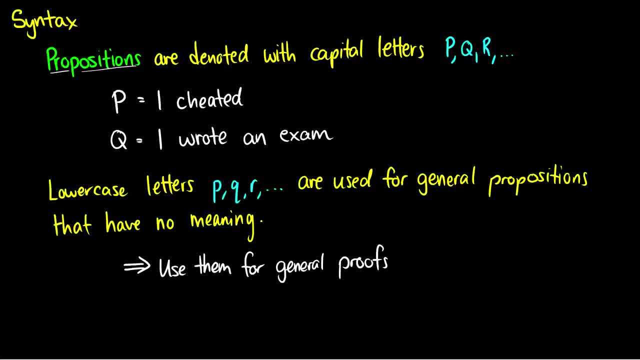 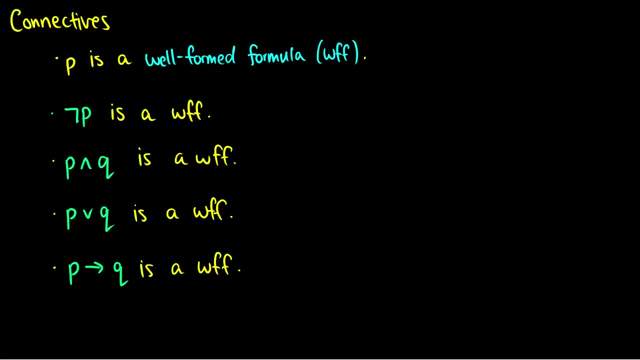 general propositions that don't have any specific meaning, And we'll be using these for proofs. So capital letters will have English translations, while lowercase letters will not. Now, with all of these different propositions, we can use connectives to change their meaning or combine their meanings together. So the first. 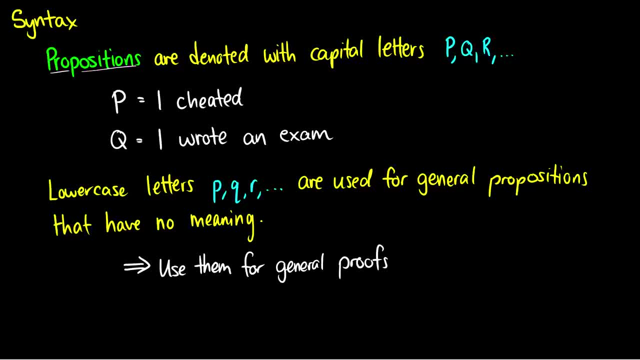 of a statement, But for this course that really doesn't matter at all. The distinction isn't important. If you're a philosophy of logic instructor or a student, then it might be a little bit important to distinguish between the two. But propositions or statements are going to. 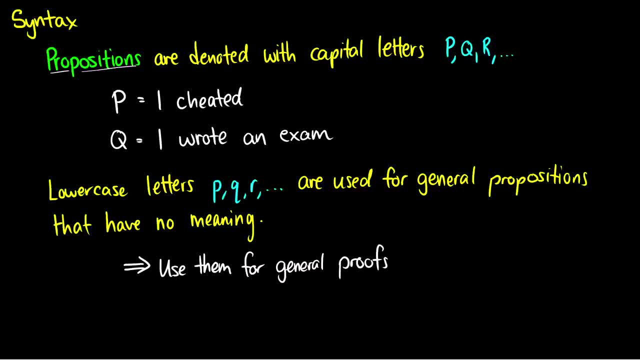 be denoted with capsules. So if you're a philosophy of logic instructor or a student, then you're going to be denoted with capital letters like PQR. So, for instance, P is I cheated and Q is I wrote an exam. So those are propositions. Lowercase letters P, Q and R are just. 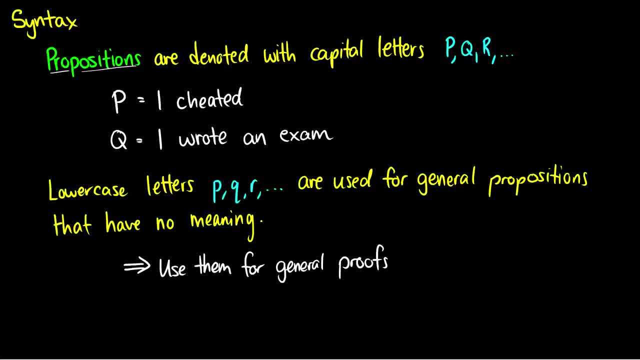 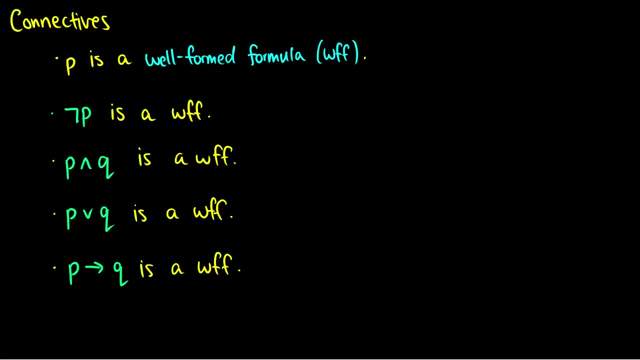 general propositions that don't have any specific meaning, And we'll be using these for proofs. So capital letters will have English translations, while lowercase letters will not. Now, with all of these different propositions, we can use connectives to change their meaning or combine their meanings together. So the first. 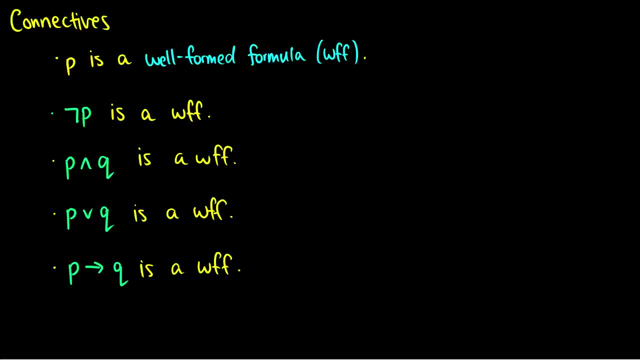 thing I want to say is that a statement or proposition on its own is a well-formed formula, also known as a WFF or a woof, which means that it is okay in our syntax. The second statement says that NOT P is a woof. So if P is a woof, then NOT P is a woof, And this NOT just means negation. So this little. 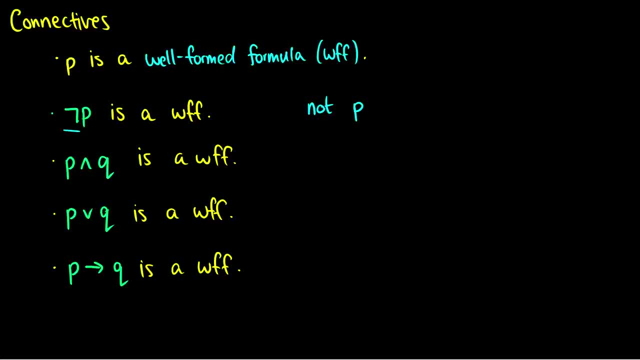 half of a box is just NOT. The second one says that P AND Q is a woof. So if P is a woof and Q is a woof, then we can connect them together for P and Q as a woof, And this is also known as a carrot. That is the. 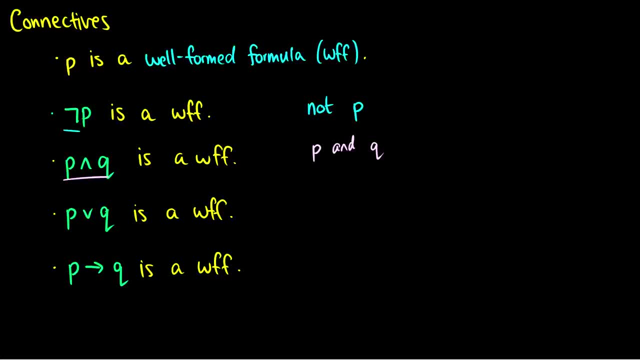 AND symbol. that is a carrot. Third: P OR Q is a woof. So this is P OR Q, And sometimes you might just call it P-V. So this is P OR Q, and sometimes you might just call it P-V. 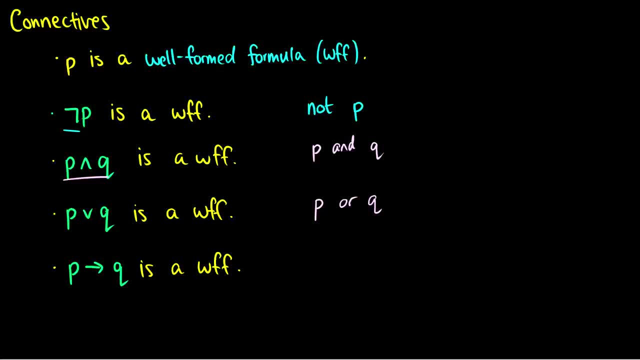 So this is P OR Q, And sometimes you might just call it P-V, And sometimes you might just call it P-V, VQ or P, wedge Q. And finally the fifth one: P, arrow Q. or rather, if P, then Q is a woof. 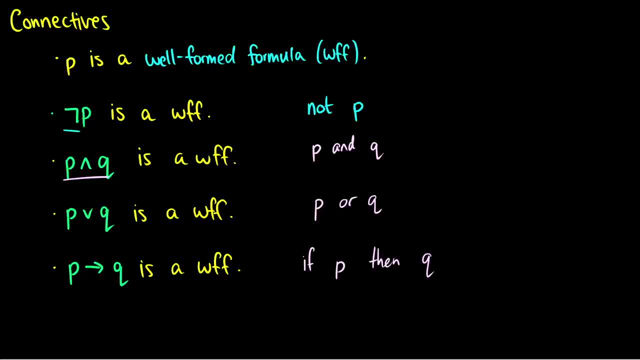 So if we have a proposition we can do not P, we can do P and Q. we can do P or Q and then we can also do: if P, then Q, And when we get to the truth tables video, we'll learn about the truth. 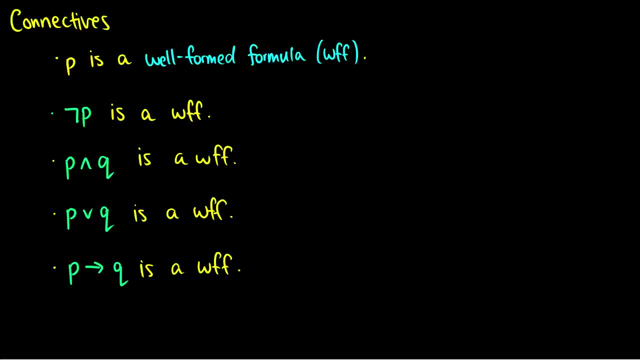 thing I want to say is that a statement or proposition on its own is a well-formed formula, also known as a WFF or a woof, which means that it is okay in our syntax. The second statement says that NOT P is a woof. So if P is a woof, then NOT P is a woof, And this NOT just means negation. So this little. 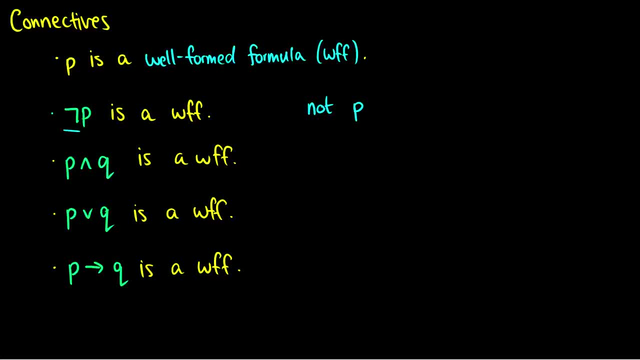 half of a box is just NOT. The second one says that P and Q is a woof. So if P is a woof and Q is a woof, then we can connect them together for P and Q as a woof, And this is also known as a carrot. 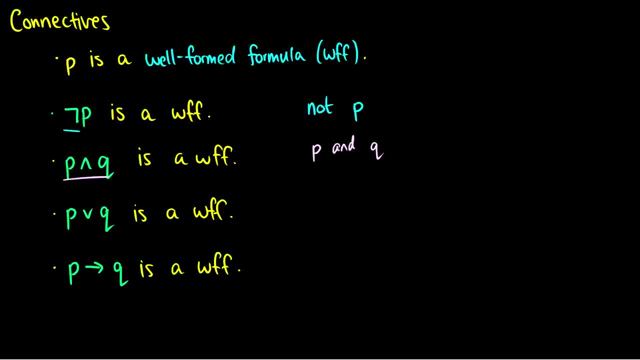 That is the and symbol. that is a carrot. Third, P or Q is a woof. So this is P or Q, And sometimes you might just call it P, V, And sometimes you might just call it P or Q. And sometimes you might just call it P or Q And sometimes you might just call it P or Q. 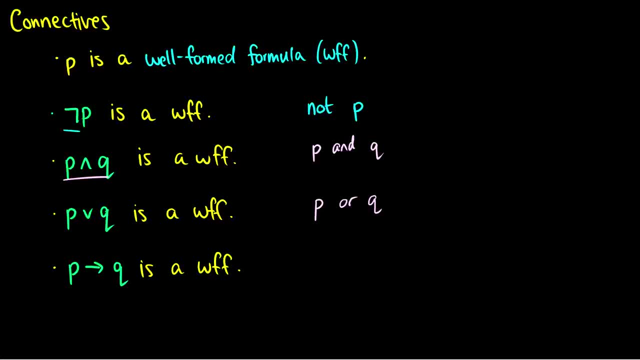 VQ or P, wedge Q. And finally the fifth one, P arrow Q. or rather, if P, then Q is a woof. So if we have a proposition, we can do not P, we can do P and Q, we can do P or Q, and then we can. 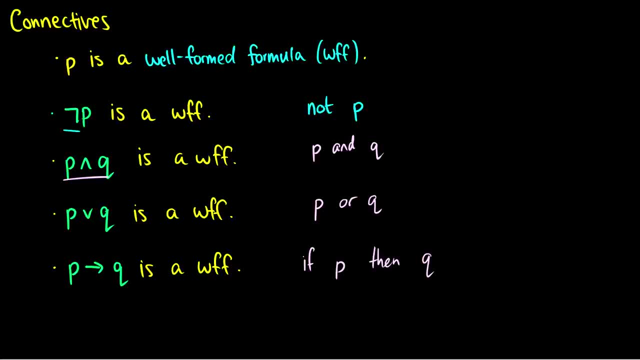 also do. if P, then Q, And when we get to the truth tables video, we'll learn about the truth conditions of each of these and how the truth output changes depending on the truth value of the propositions. But for now, I just want to focus on translating these into English. So here: 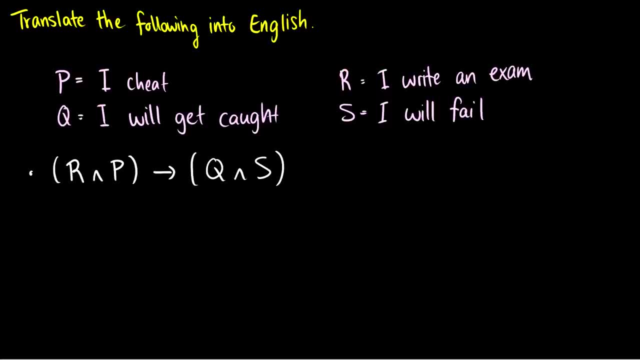 is a key of propositions, And here is a well formed formula And I'm saying: translate the well formed formula into English. So I am just going to read this out. So R and P, arrow, Q and S, And this can be translated to: if R and P. 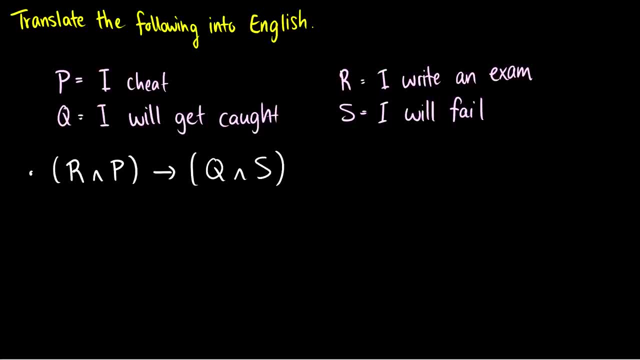 then Q and S. So how can we translate this into English? Well, let's do the arrow in a color, So we have, if a bunch of stuff, then some more stuff, And let's do the first bit first. So this is, and with the conjunction, So what is R? 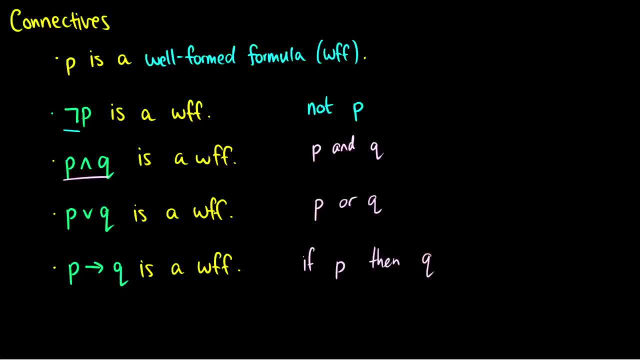 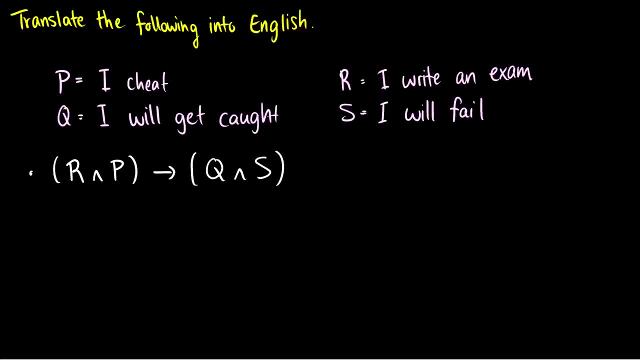 conditions of each of these and how the truth output changes depending on the truth value of the propositions. But for now I just want to focus on translating these into English. So here is a key of propositions And here is a well formed formula. And I'm saying: translate the. 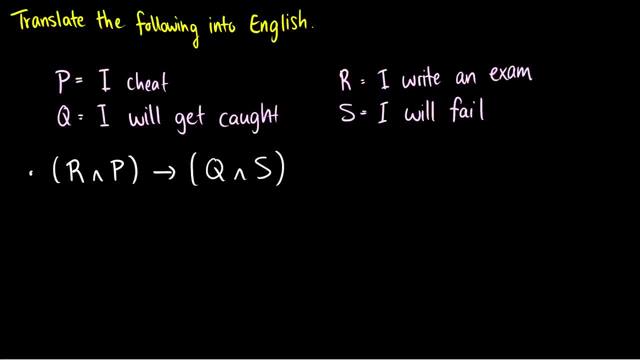 well formed formula into English, So I am just going to read this out. So R and P, arrow, Q and S. And this can be translated to: if R and P, then Q and S. So how can we translate this into English? Well, let's do the arrow in a color. 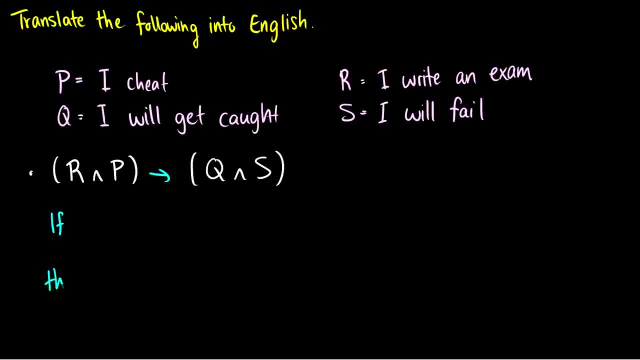 So we have, if a bunch of stuff, then some more stuff, And let's do the first bit first. So this is, and with the conjunction: So what is R? Well, R is if I write an exam, and then we have our connective and And now we have P. So what is? 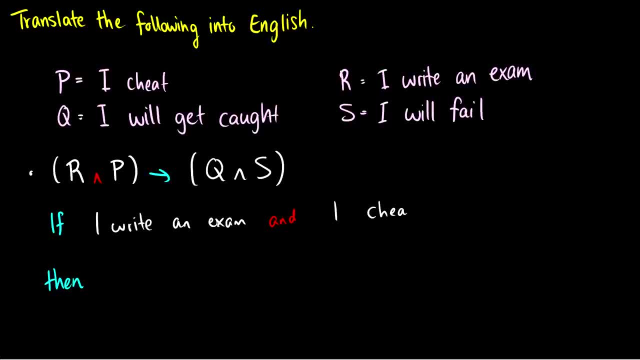 P. Well, P is I cheat. So if I write an exam and I cheat, then with the arrow Q, so I will get caught, And then with the arrow Q I will get caught. Then with the arrow Q, I will get caught, And then with the arrow Q, I will get caught. 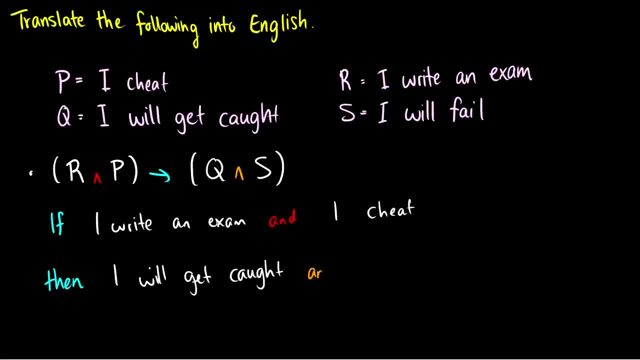 Then with the arrow Q, I will get caught, And then with the arrow Q, I will get caught. This, and which I'll just rewrite in orange is also: and Then what is S? S is I will fail. So this well formed formula, given the key above, translates into: 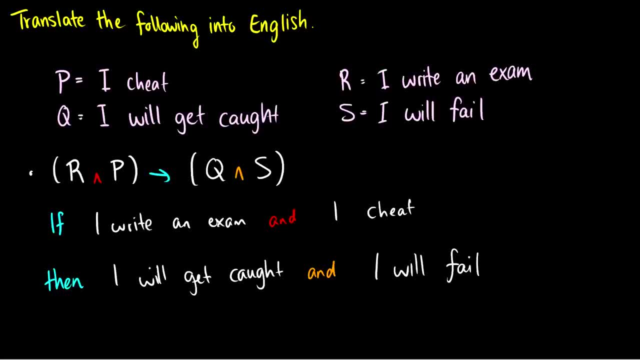 if I write an exam and I cheat, then I will get caught and I will fail And we can kind of see the groupings here. So we can see that R and P are grouped together and Q and S is a group together. So we can see that R and P are grouped together and Q and S is a group together. 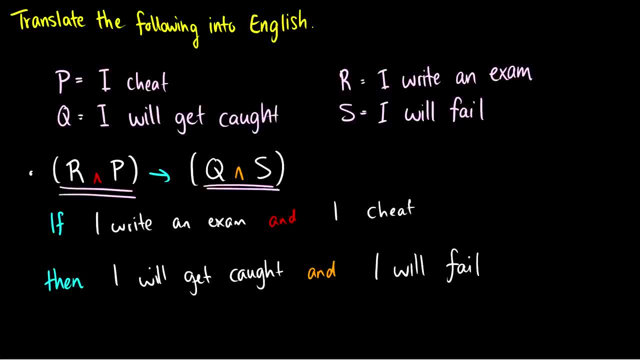 So if R and P, then I will fail p, then q and s, and all i did was translate this well-formed formula into english, given the keys above. of course. if i changed what the keys meant, then of course the sentence would change as well. in fact, it's not important that our sentence makes any sense at all, so these keys just happen to. 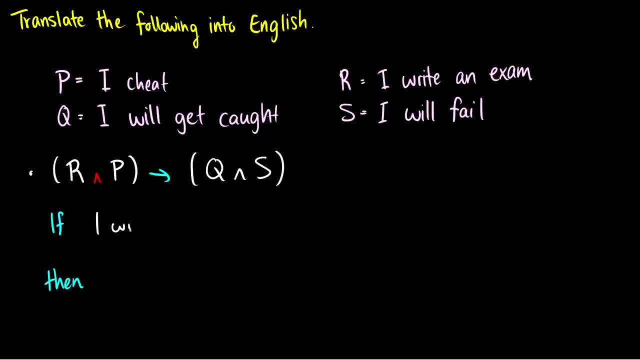 Well, R is if I write an exam and then we have our connective and And now we have P. So what is P? Well, P is I cheat. So if I write an exam and I cheat, then with the arrow Q, so I will get caught. 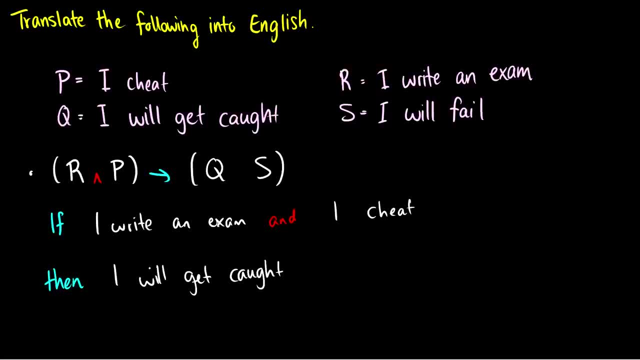 And then with the arrow Q, I will get caught, Then with the arrow Q, I will get caught, And then with the arrow Q, I will get caught. And this, and which I'll just rewrite in orange is also: and Then what is S? S is I will fail. 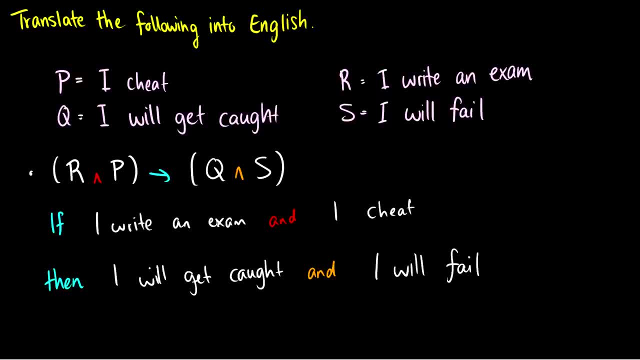 And this well formed formula, given the key above, translates into: if I write an exam and I cheat, then I will get caught and I will fail, And we can kind of see the groupings here. So we can see that R and P are grouped together And Q and S is a group together. So if R and P, then P and S are related. Then if I write an exam and I cheat, then I will get caught And we can see the groupings here. So we can see that R and P are grouped together And Q and S is a grouped together. 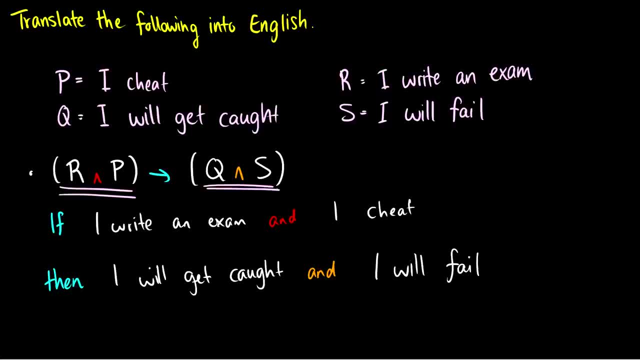 p, then q and s, and all i did was translate this well-formed formula into english, given the keys above, of course. if i changed what the keys meant, then of course the sentence would change as well. in fact, it's not important that our sentence makes any sense at all, so these keys just happen to. 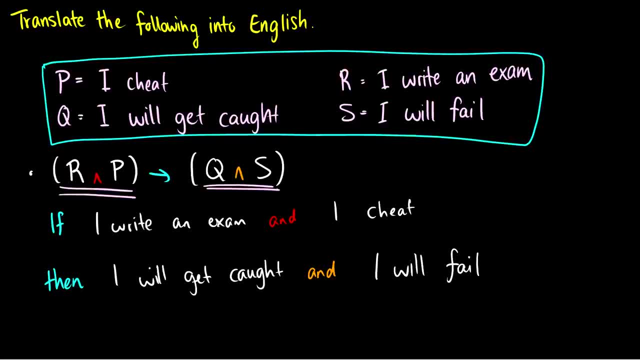 make a sentence that made sense, but it doesn't have to make sense, so keep that in mind when doing some of the problems on your own, because it's not always the case that what you translate is going to make much sense at all. now that we've done a well-formed formula into english, 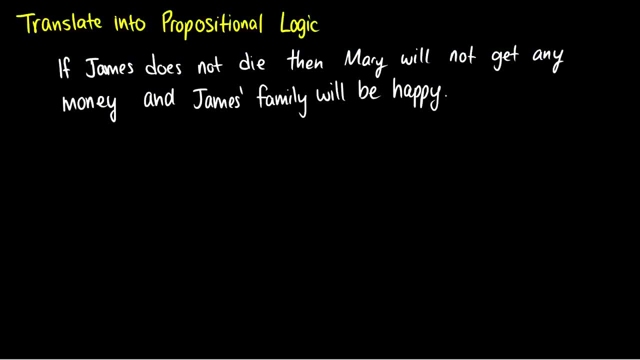 let's do english into a well-formed formula. so i have this sentence here: if james does not die, then mary will not get any money and james family will be happy. so the first thing i kind of want to do is look at all the connectives. so the first thing i see here is an if then statement. 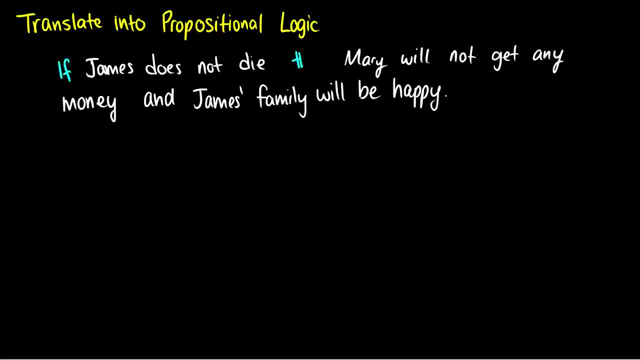 sorry, i'm going to rewrite this if and then in light blue, which means at some point we're going to need an arrow if james does not die. oh, i see a knot in here, so let me put that in red. then mary will not get any money. i see another knot there. that is another connective. and oh, there's an. 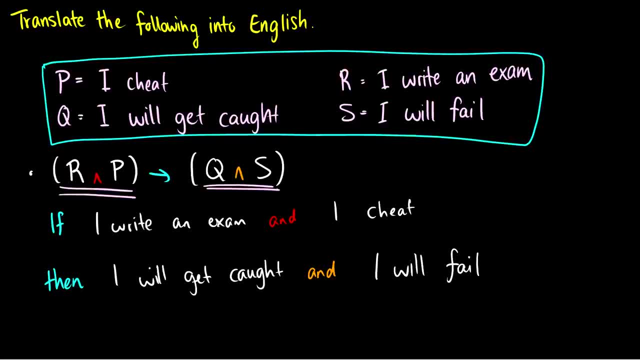 make a sentence that made sense, but it doesn't have to make sense, so keep that in mind when doing some of the problems on your own, because it's not always the case that what you translate is going to make much sense at all. now that we've done a well-formed formula into english, 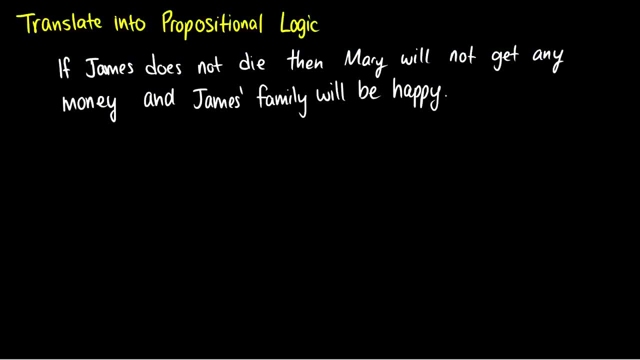 let's do english into a well-formed formula. so i have this sentence here: if james does not die, then mary will not get any money and james family will be happy. so the first thing i kind of want to do is look at all the connectives. so the first thing i see here is an if then statement. 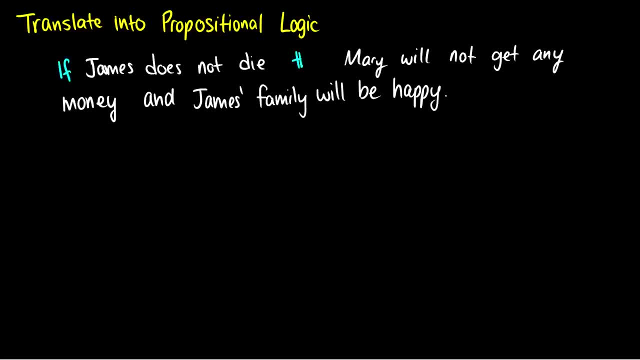 sorry, going to rewrite this if and then in light blue, which means at some point we're going to need an arrow if james does not die. oh, i see a knot in here, so let me put that in red. then mary will not get any money. i see another knot there and that is another connective. and oh, there's an. 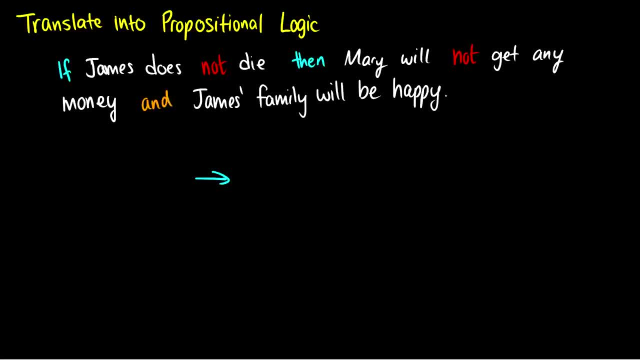 and so let's do, and in orange, james family will be happy. so what i see here is i see an. if then statement with James does die, with a not in there, so we're going to have not something, then Mary will not get any money, so there's a not there, and then there's something else, so it looks like 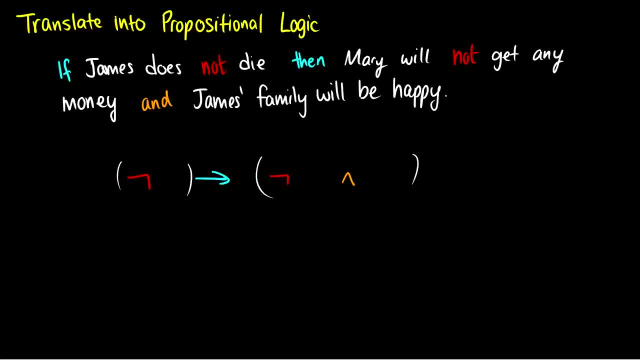 our translation is going to take this form. now we just have to define our keys. so the first key would be: James does die or James dies. so we can call this: p is equal to James dies. now why can't we say p is equal to James does not die? well, not is a connective. so when we translate or give a key, 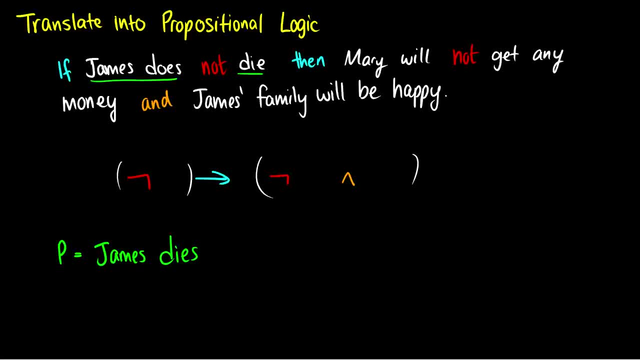 for our propositions. we want them to be an affirmative or a positive statement. we want not to be a connective that attaches to an affirmative statement. you. so if p is James dies, then not p would be: James does not die, so the next one, then the next proposition- Mary will get any money- would be another statement or proposition. 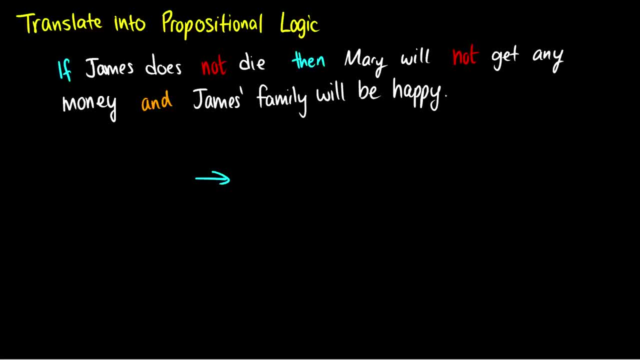 and so let's do, and in orange, james family will be happy. so what i see here is i see an then statement with James does die, with a not in there, so we're going to have not something. then Mary will not get any money, so there's a not there, and then there's something else, so it looks like 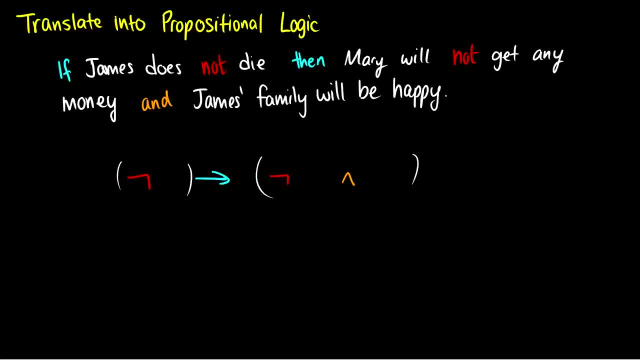 our translation is going to take this form. now we just have to define our keys. so the first key would be: James does die or James dies. so we can call this: p is equal to James dies. now why can't we say p is equal to James does not die? well, not is a connective. so when we translate or give a key, 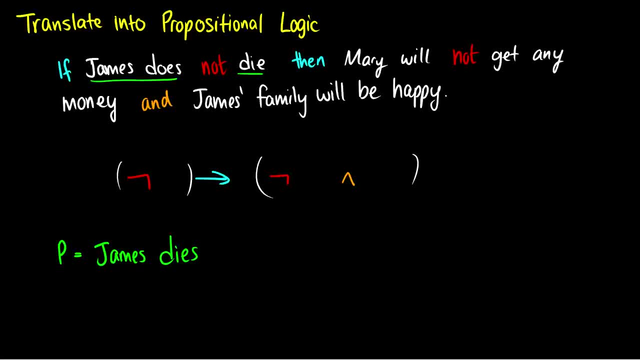 for our propositions. we want them to be an affirmative or a positive statement. we want not to be a connective that attaches to an affirmative statement. you. so if p is James dies, then not p would be: James does not die, so the next one, then the next proposition- Mary will get any money- would be another statement or proposition. 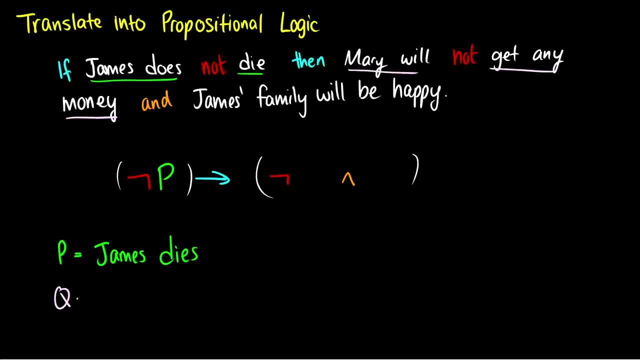 we wouldn't include not in there. so let's call that q. Mary will get money and I know it says we'll get any money. but the way that not works in English is we kind of need to make sure that it's not attached to not. if we say Mary will get any money, that sounds weird in. 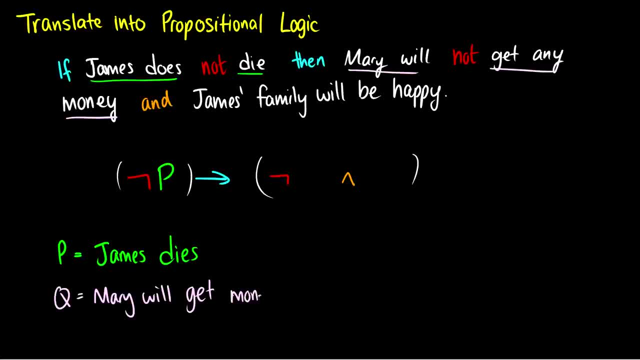 English, so we just kind of alight it. so Mary will get money, so it'll be not q and finally James family will be happy. so we can call this r, define this as James family will be happy, and then finally, we can stick this into our last slot r. 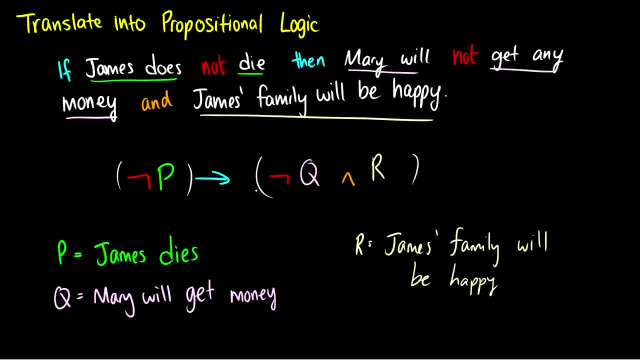 so if not p, then not q and r, and when we just have one statement on its own, we can just remove the brackets. so this says: if it is not the case that James dies, or if James does not die, then it is not the case that Mary will get money and James family will be happy. so 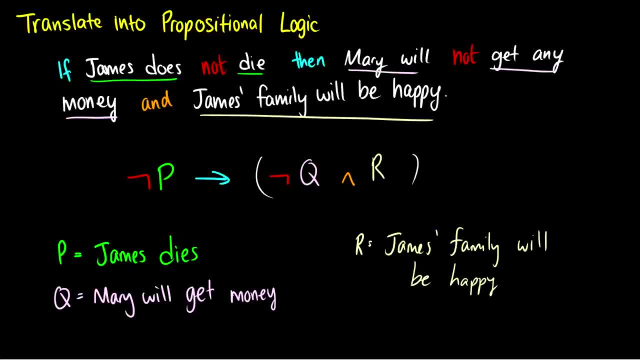 hopefully, with these examples, you kind of see how to take an English sentence and translate it back into a well-formed formula, and vice-versa. so I did put this out there. if you have any questions or questions, please feel free to use my staff at the end of my video.